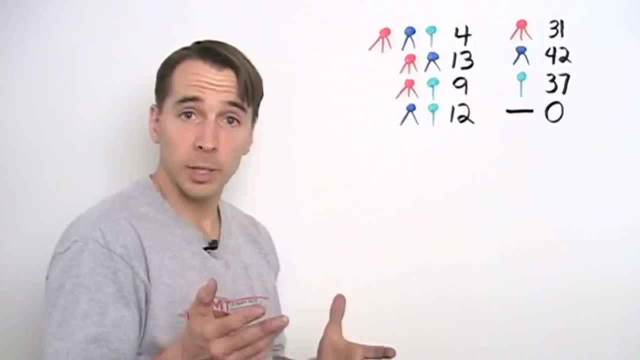 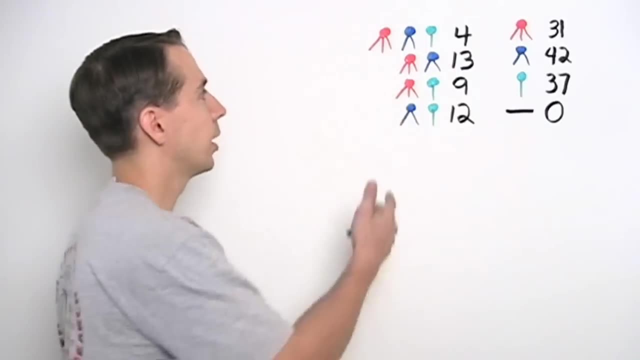 37 of these green one-tasseled ribbons. Now some of the dogs received more than one ribbon. Four super dogs got all three and there were 13 who got a red and a blue. that includes all the super dogs. 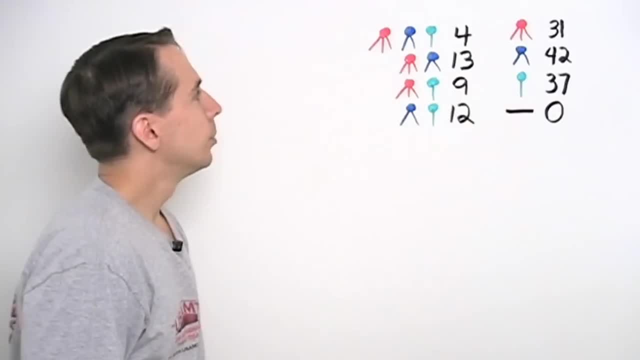 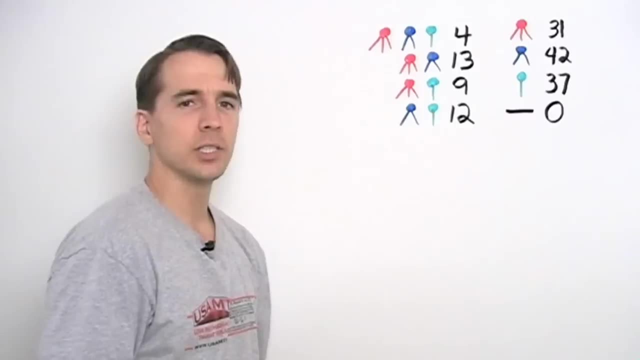 and nine who got a red and a green, four who got a blue and a green. But you know I wasn't really concerned about the prizes. You know, counting the ribbons that's not hard. I can just add all these up. 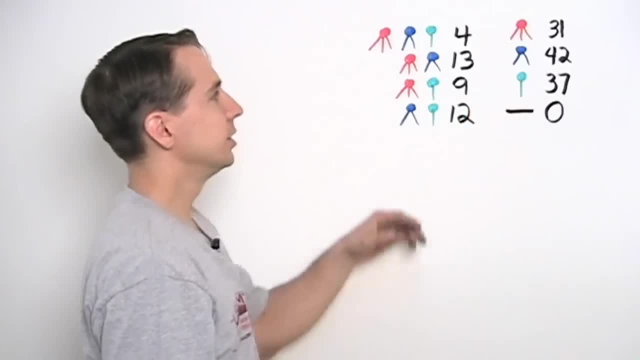 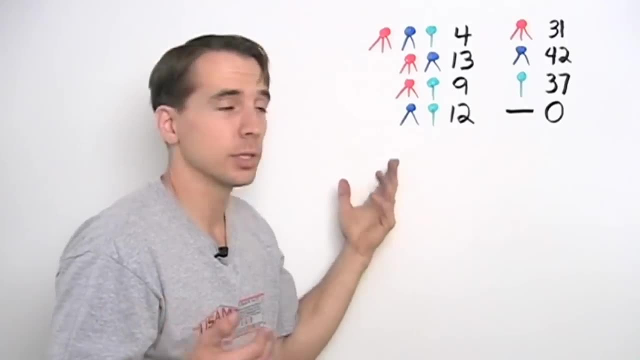 But I wanted to know how many dogs there were, and I can't just add these three up, Because if I just add the red, the blue and the green ribbons that were given out, I'm going to count the super dogs three times. I'm going to count some of these other dogs twice. 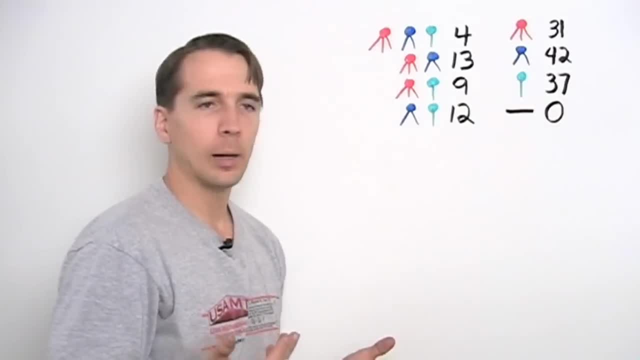 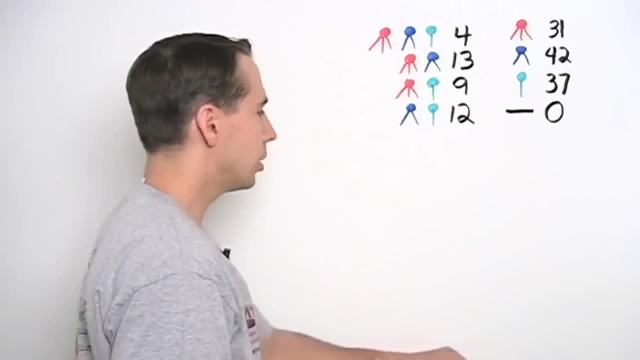 So I can't just add these three numbers up to figure out how many dogs there were. Well, I like the dogs a lot more than the prizes, So I wonder how many dogs are here? I figured. I'll try my Venn diagram. 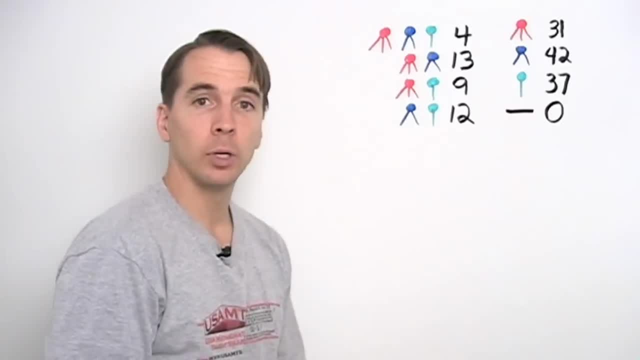 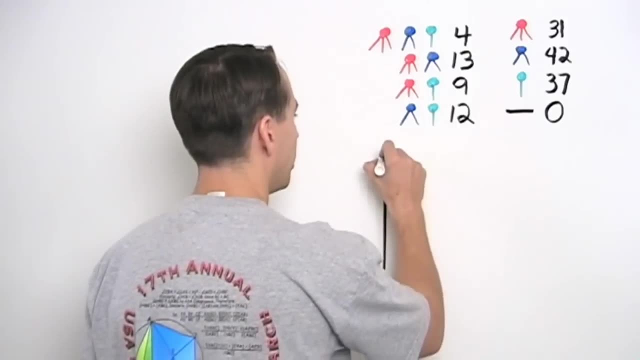 Except I'll try three circles: one green, one blue, one red, one for each ribbon instead of just two. So we'll start off with a box. Put all the dogs, all the dogs go in a box. That way they can't run around as much and they'll be easier to count. 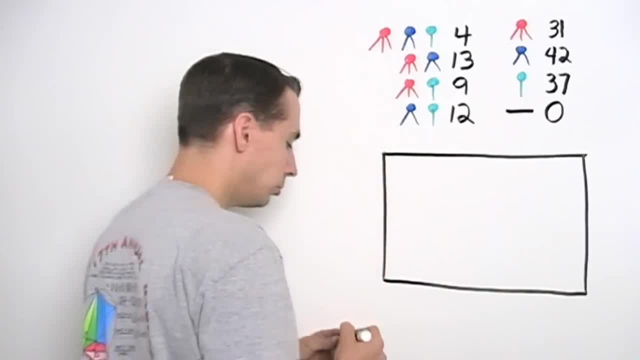 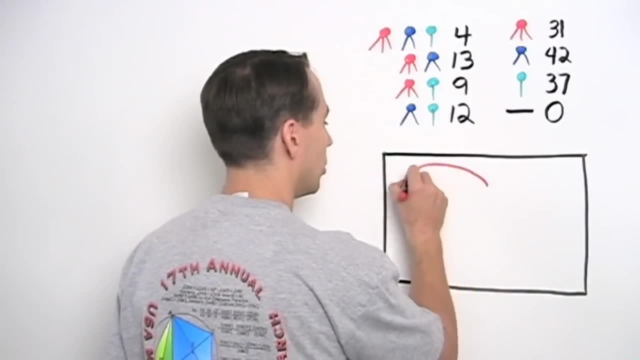 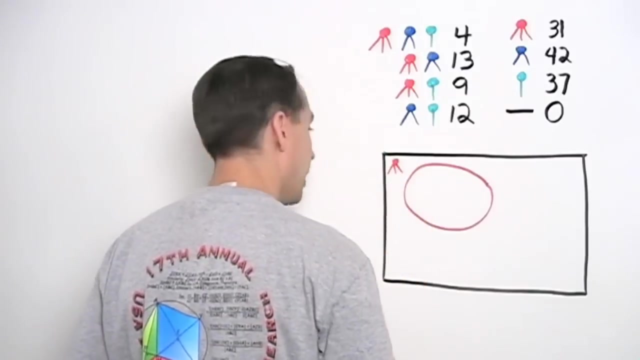 So there's our box. We're going to have one circle for each ribbon, So we'll start with a red ribbon And all the dogs who want a red ribbon go in the red circle, And then next green, All the dogs. 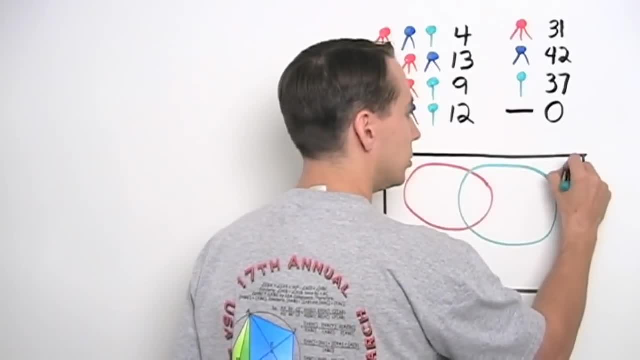 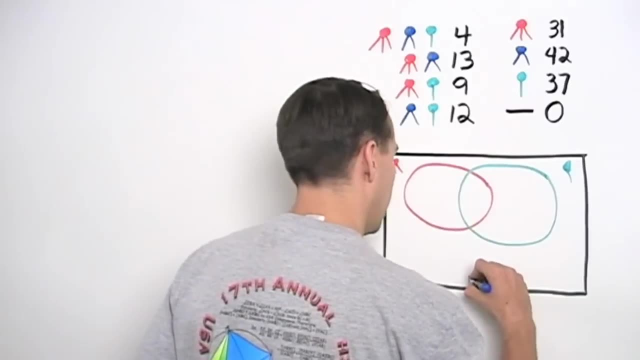 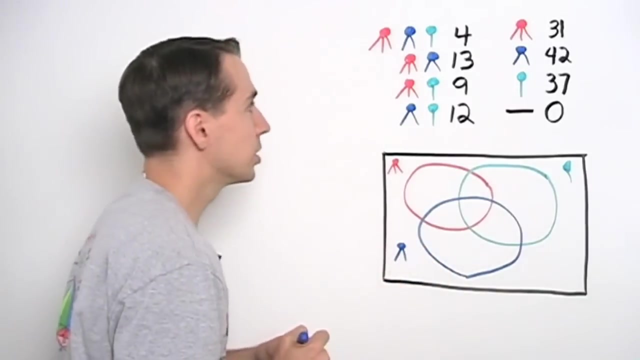 who want a green ribbon go in the green circle, And then all the dogs who want the two tassel blue ribbon, they go in the blue circle And now all you have to do is take the dogs, put them in the right place in the box. 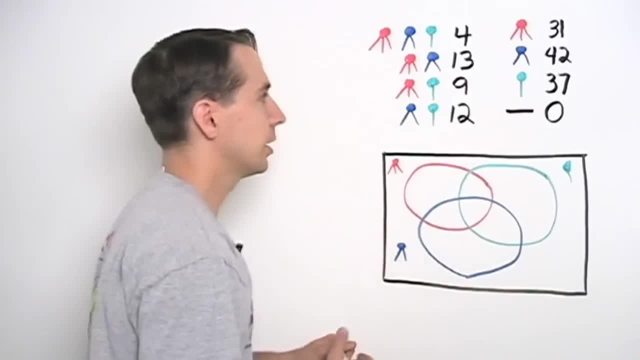 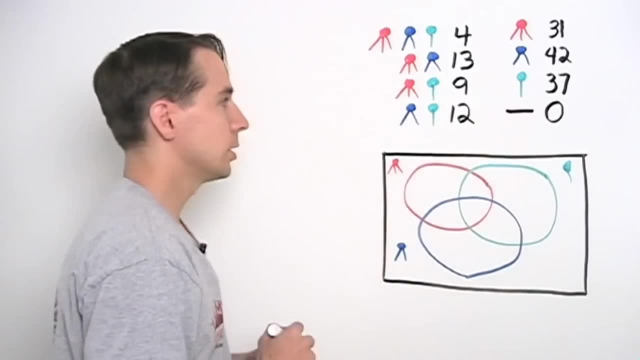 Now we'll start with the outside, because that's easiest. There are no dogs who are very concerned about the self-esteem of the poor little doggies, Or at least the poor little doggie owners. There were no dogs who received no ribbons. 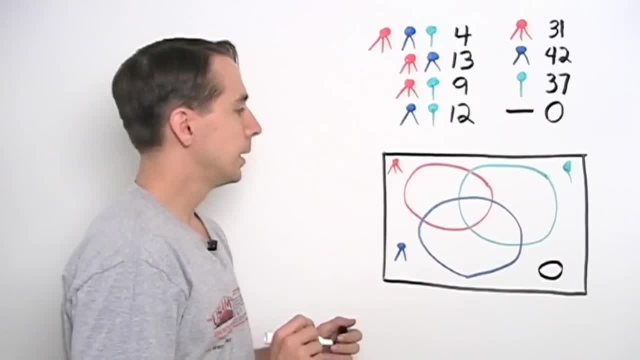 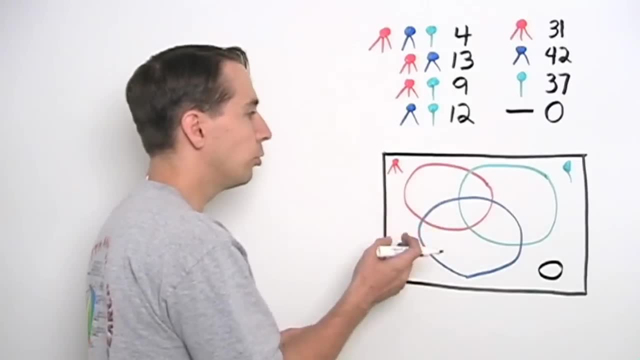 So there are no dogs sitting out here. Now what Well? we can't start here with the dogs that received red ribbon and nothing else, Because we don't know that number. All we know is that there are 31 in this whole circle. 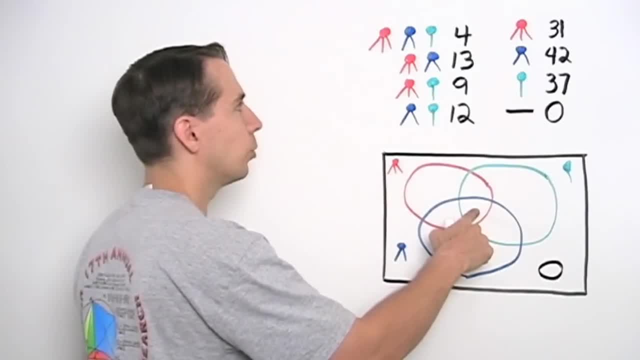 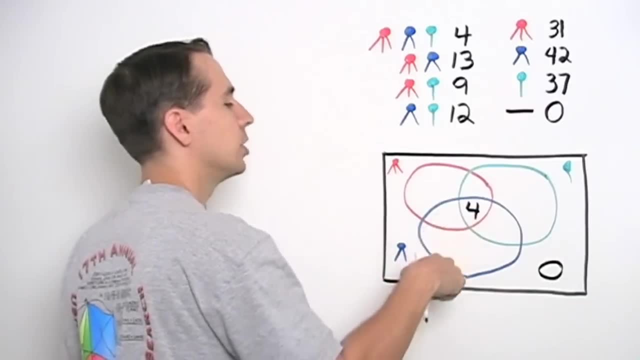 But we do know if we start from the middle, start from the inside and work out, well, we do know there are four super dogs And they're the dogs that are in all three circles. So this overlap region where all three circles overlap, 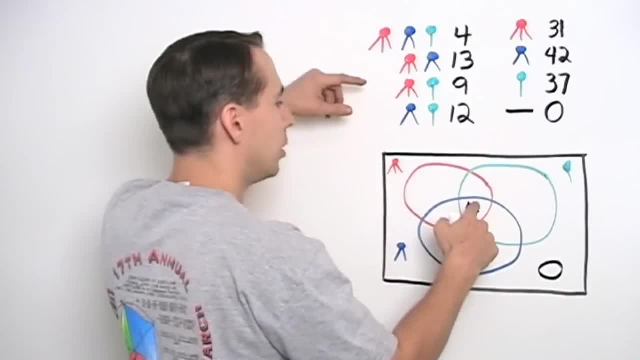 there are four, And once we have that, now we can work from the inside out And let's see. we'll start here. There are 13 with red and blue, so there are 13 in the overlap of red and blue. 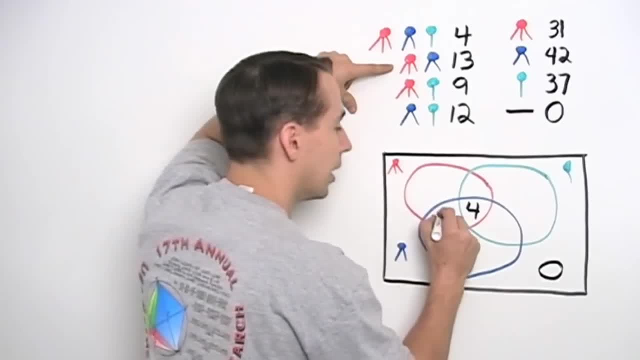 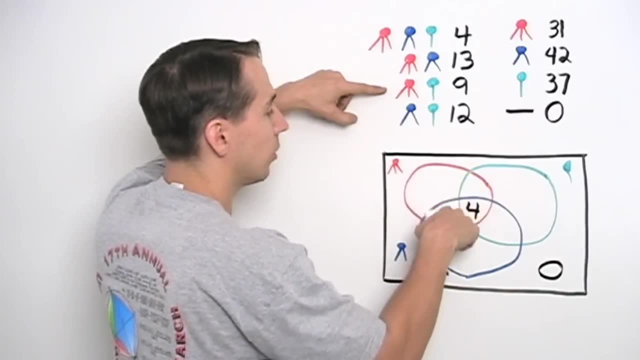 We already have four super dogs here, so there have to be nine out here. Those nine got a red and a blue and not a green, And in just the same way we look at the red and green overlap, there should be nine total. 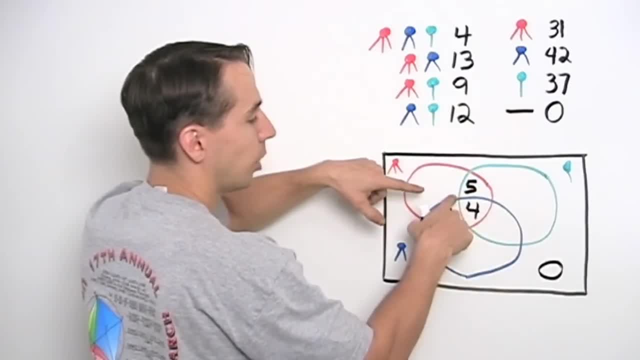 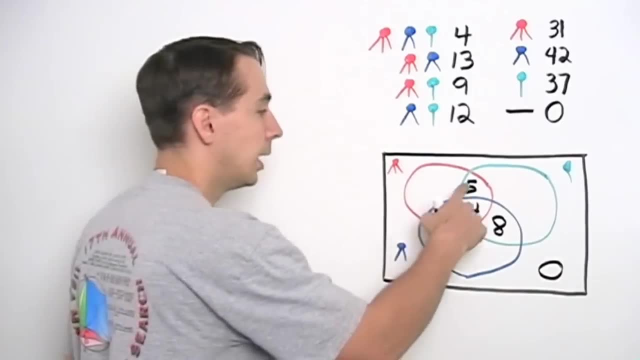 We have four accounted for, so there are five out here. There have to be 12 in here. We have four accounted for, so there are eight that received a blue and a green but no red. Now that we have these three numbers, 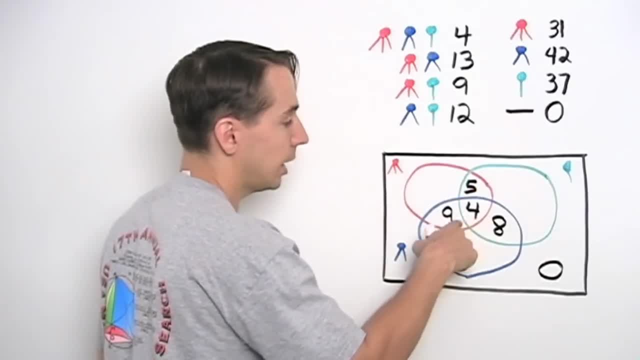 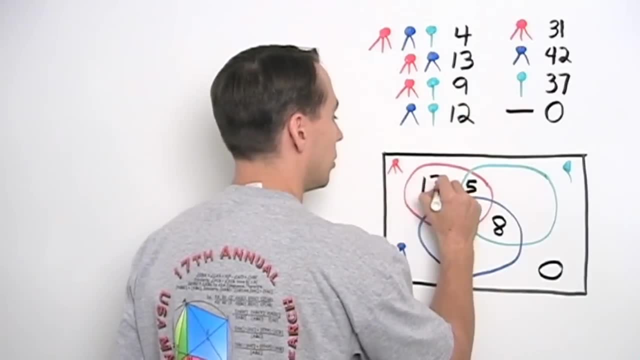 we can figure out how many received only red. We've already counted 18 dogs that have received a red ribbon. There are 31 total. that leaves 31 minus 18, so 13 dogs received a red ribbon and nothing else. 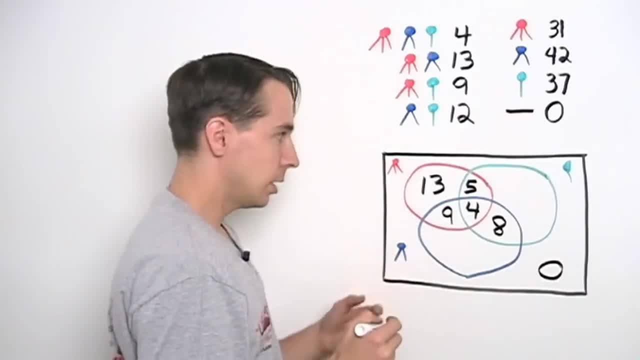 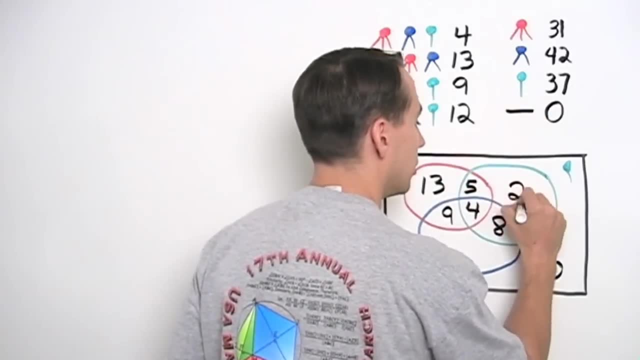 And then over here we've counted five plus four plus eight, so nine plus eight is 17.. 17 green ribbons have already been accounted for, so 37 minus 17 leaves 20 dogs who received only a green ribbon. 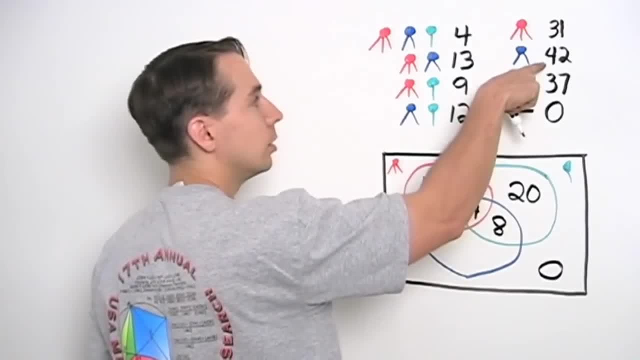 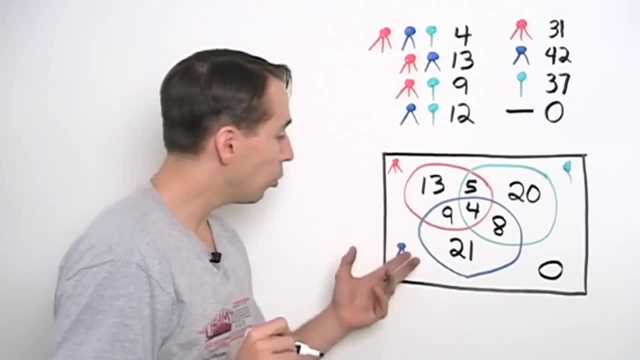 And finally, eight plus four is 12, plus nine is 21.. There are 42 blue ribbons given out total, so there are 21 dogs who only received a blue ribbon. And now we can tally up the dogs, So let's go ahead and count them up. 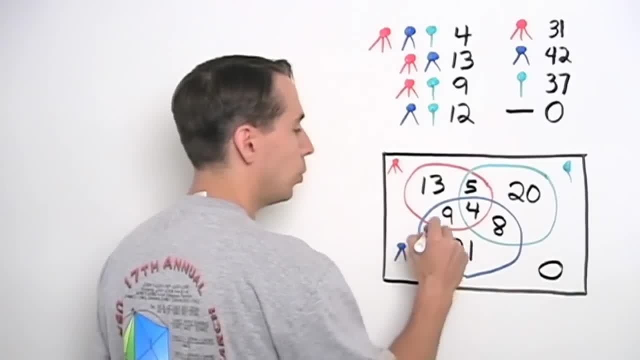 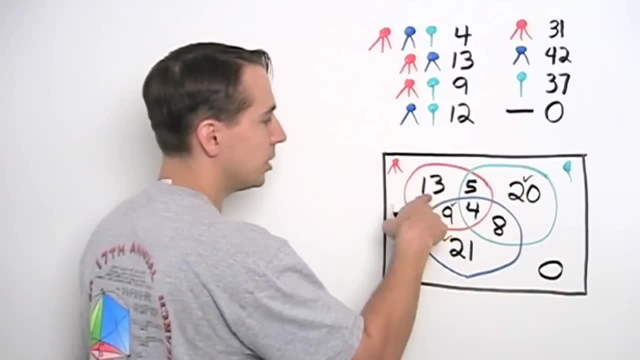 I'm going to kind of group them by tens to make it a little easier to count. We've got 21 plus nine, that's 30, plus our 20 over here is 50. Now when we add up these, well, we have 13 plus five is 18,. 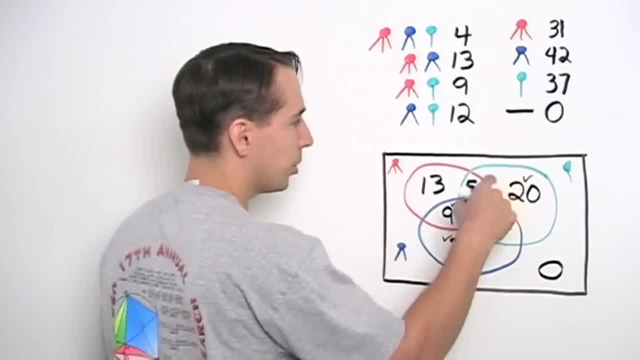 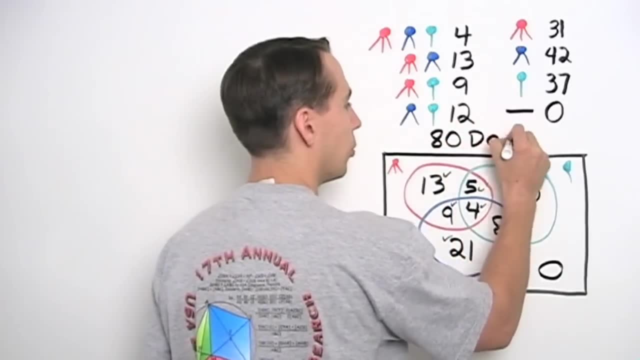 plus four is 22,. plus eight is 30.. 30 plus the 50 we already had- check them off as I count them- gives us 80 dogs Total. And there we go. I've counted the dogs. Use the Venn diagram. 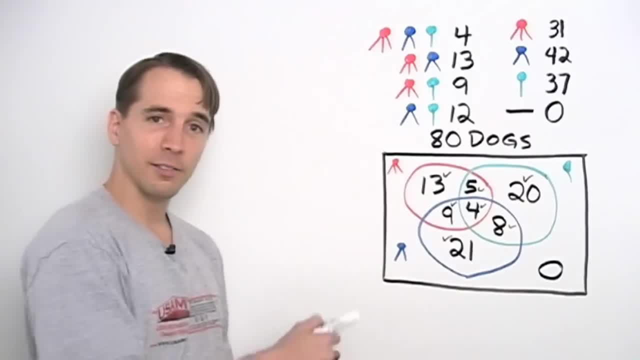 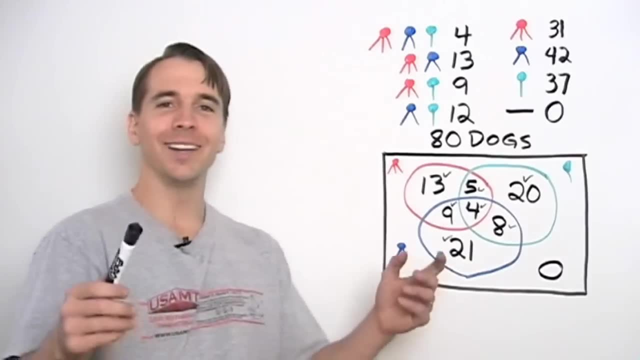 I thought that was really slick. I showed it to my friend John. I said, hey, Venn diagram, three circles, Let's see your subtraction method do that. And he said, hey, that's as easy as pie. He even wrote it down. 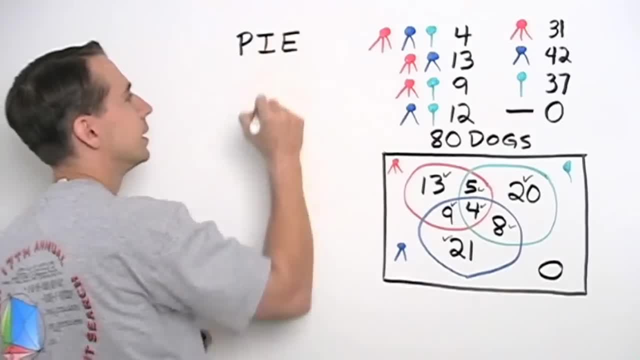 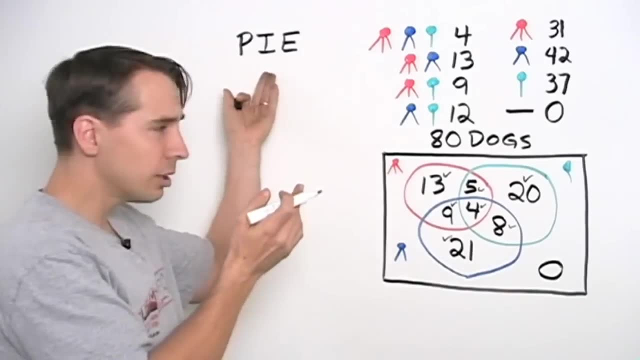 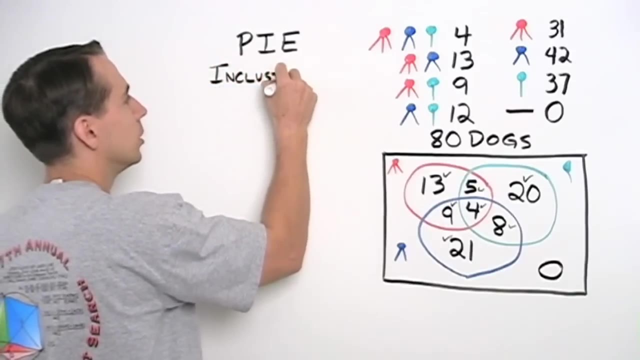 P-I-E And I said, John, that's, that's not very helpful, That doesn't tell me anything. He's like principal, inclusion, exclusion. He even wrote that down too, And then I was sure he didn't know what he was talking about. 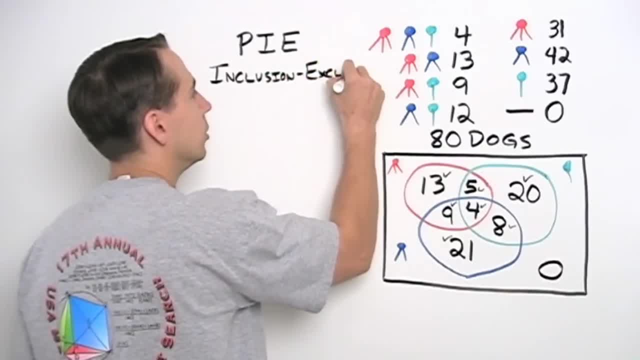 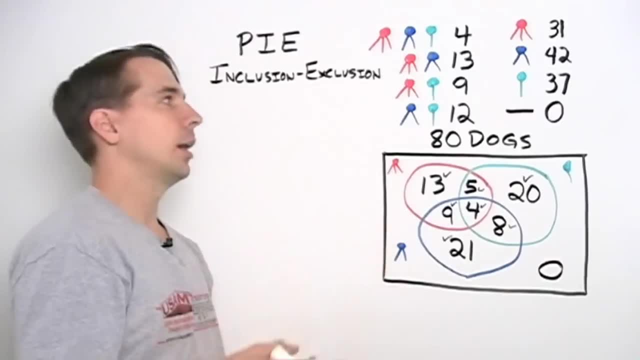 Inclusion, exclusion. I certainly didn't know what he was talking about. John, this, this doesn't help me either, You're. you're going to have to show me. And he said, okay, I'll show you how it works. 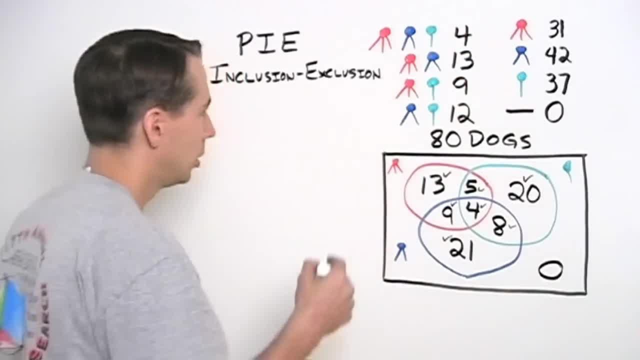 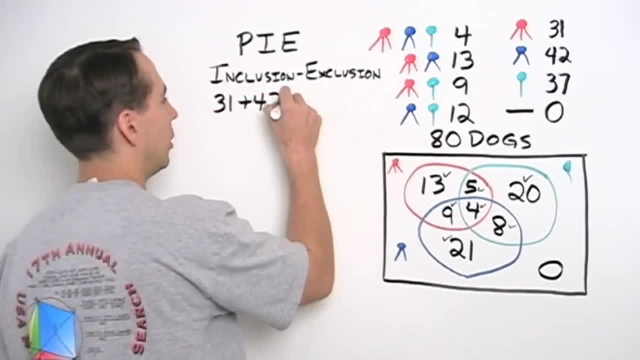 All right, we want to count the dogs, So we'll start off by counting how many ribbons are given out. He gave out 31 reds, 42 blues and 37 greens And of course I'm like come on. 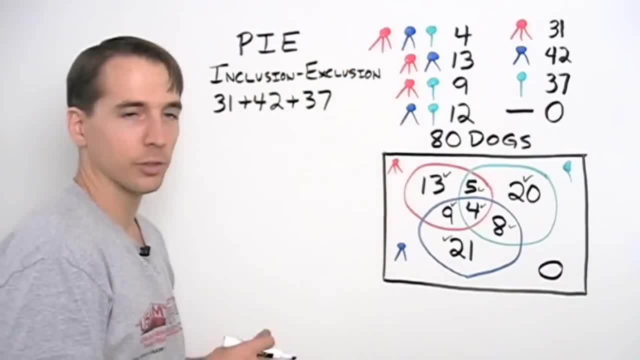 John, that's going to count some of the dogs a bunch of times. The super dogs are going to count them three times. Some of these other dogs are going to count twice. That can't possibly be right. He said, of course. 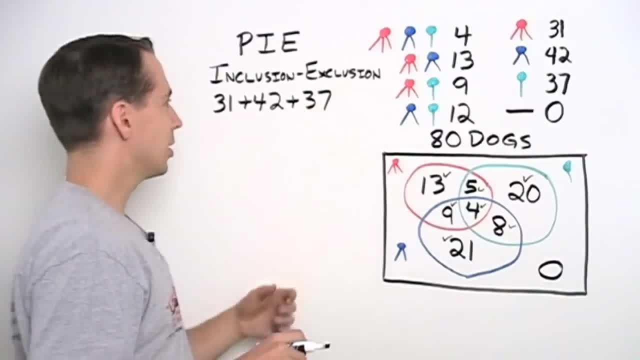 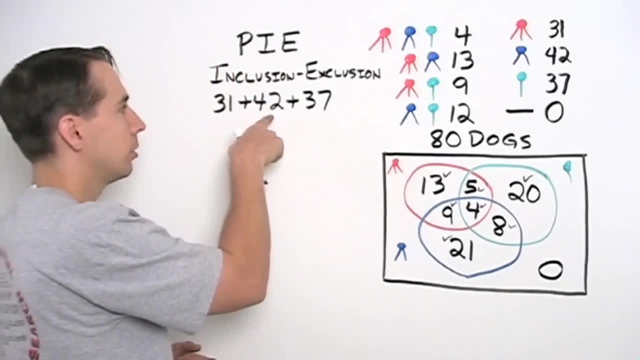 of course it's not right, Not finished. It's going to count some of these dogs twice. Let's look at the dog that gets a red and a blue ribbon. Count them once here. Count them once here. Count them twice, Only want to count them once. 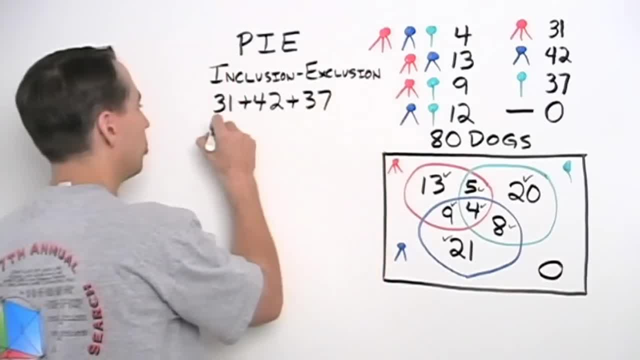 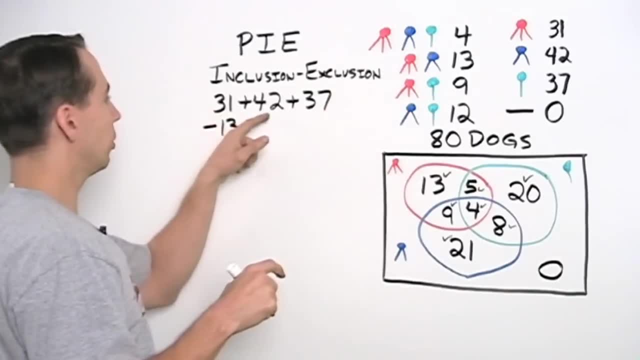 So what do we do? We subtract them once. We've counted them twice, We only want to count them once. We subtract them once. So we subtract them. Added the red and blue dog: once here, once here. Subtracted it: once here. 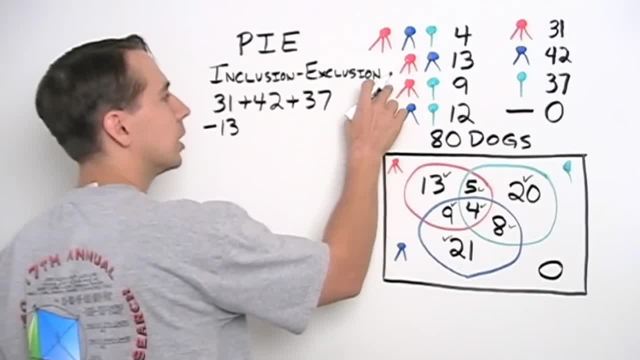 That means I've counted it once and only once. And that's the whole goal in the counting problem: Count them all once and only once. And we do the same thing with these other dogs. These dogs have got a red and a green. 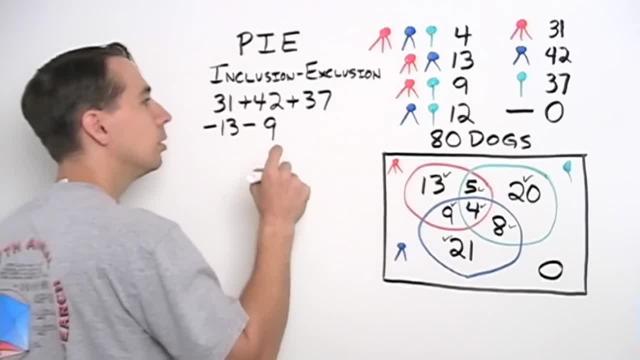 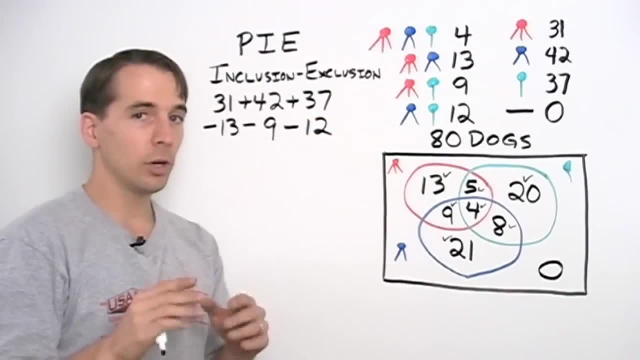 Counted them once for red, once for green, So we subtract them once for red and green. Same thing for the blue and the green dogs: Subtract them once. So now every dog that received only one ribbon is counted exactly once in one of these three. 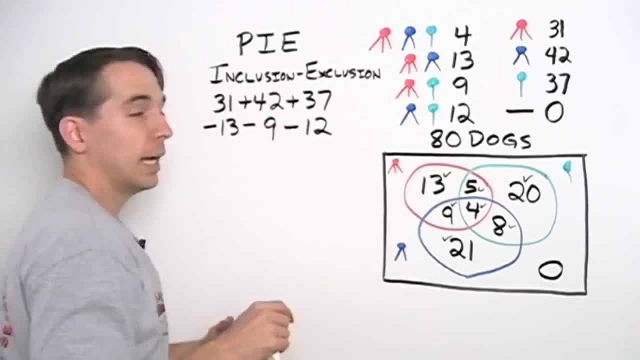 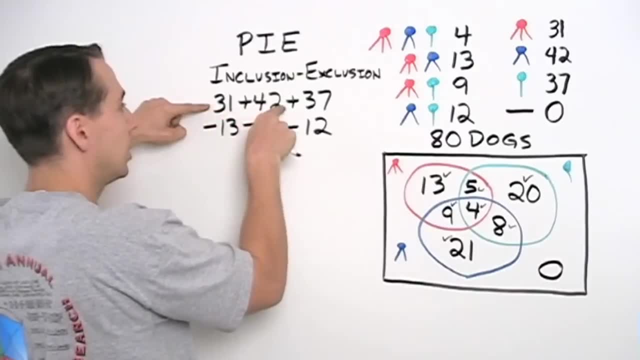 They only get a blue. They're counted here. Only get a green, Only get a red. Any dog that gets exactly two ribbons is also counted only once. Counted twice in this first line, once for each of the ribbons they get. 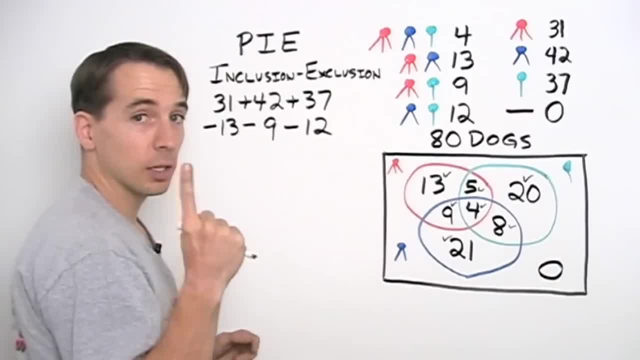 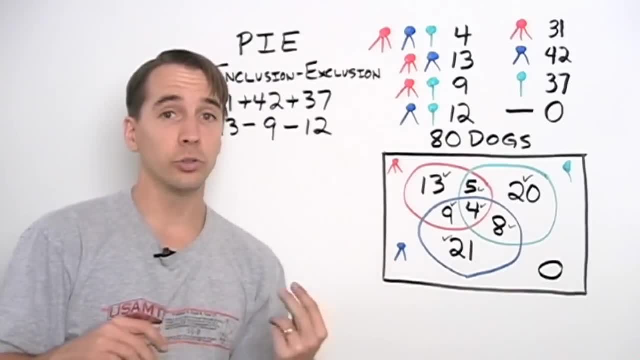 and then subtracted once. Added twice. subtracted once, That means you've counted them once and only once. So every dog that's gotten only one ribbon is counted once. Every dog that's gotten exactly two ribbons is counted once. I said: hey, John, what about the super dogs? 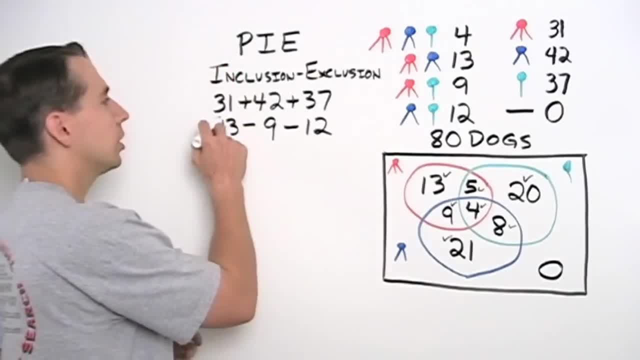 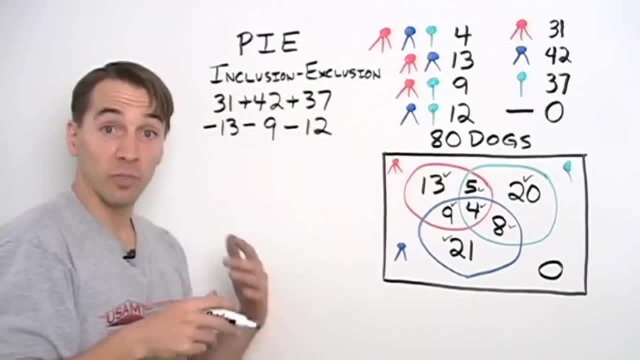 He said: hey, can't forget the super dogs. Let's take a look here at what we've done with the super dogs. Well, they're included here, so we counted them once Included here, counted them twice Included here, so we've added them three times. 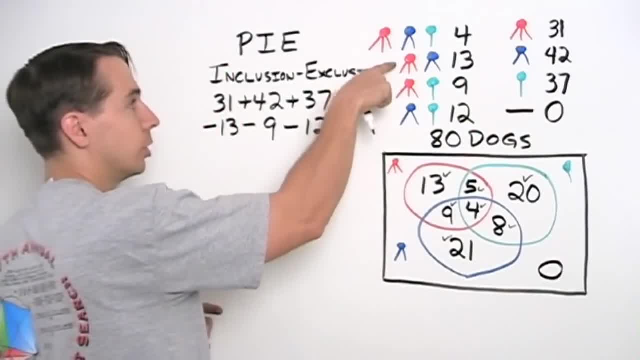 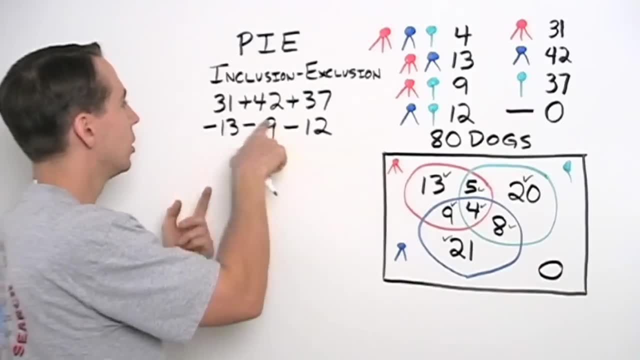 once for each of these ribbons, But each of the super dogs is also included here, here and here, Because they have these two colors, have these two colors, so we've subtracted them in each one of these, So we've added them three times. 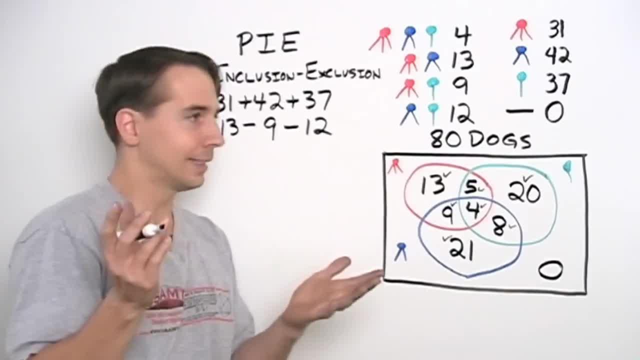 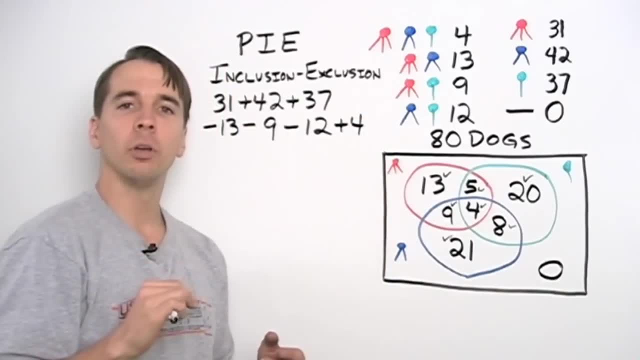 and subtracted them three times. We haven't counted them all, and you've got to count the super dogs, So we just add them back in once. And now the super dogs are counted once and only once. And sure enough, I went ahead and computed this. 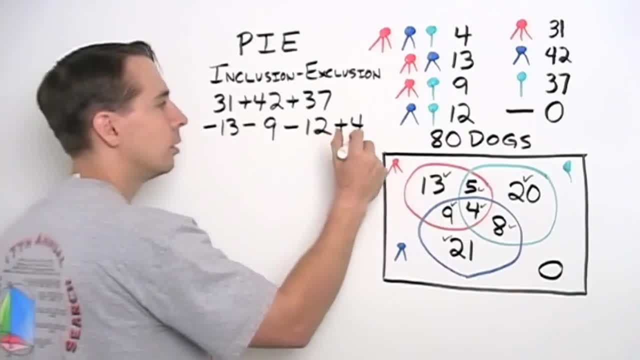 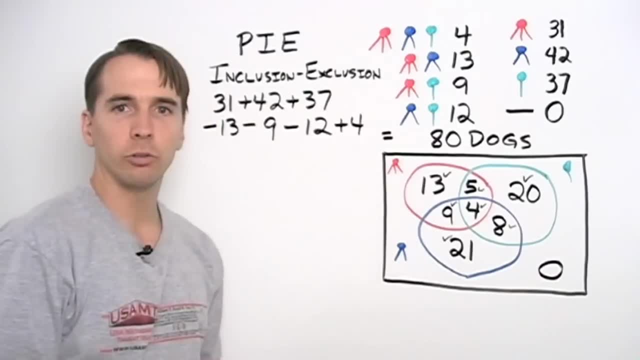 added these three, subtracted these three and added that and I got 80. It worked. This inclusion exclusion thing, this pi thing- it worked. So now we've done the problem two different ways, got the same answer. 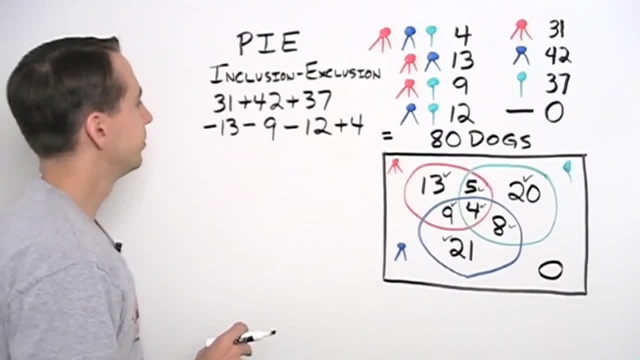 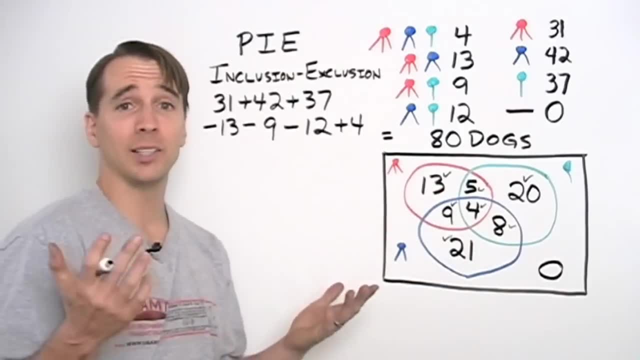 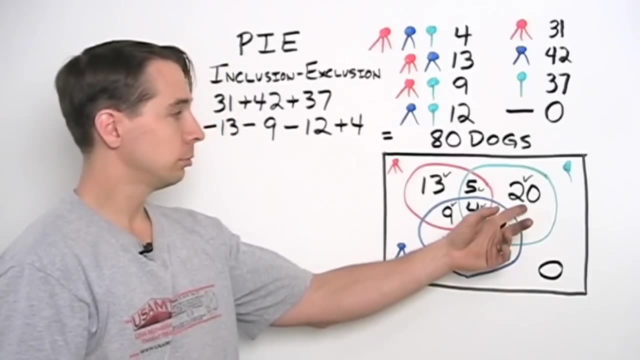 so we're pretty sure we're right. Hmm, I thought this was pretty neat, but pointing out the John Hay, look With my diagram, I can answer all sorts of other questions too. For example, how many dogs got only a green ribbon? 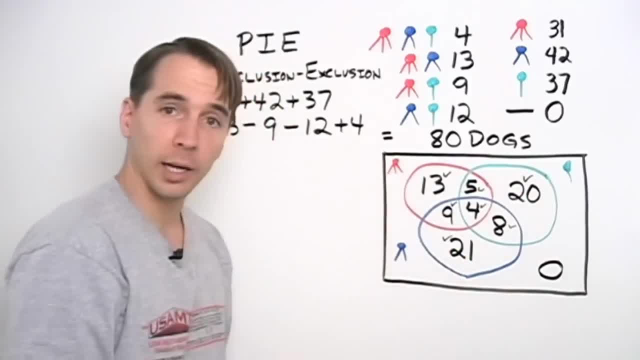 There are 20.. I see it right there on my diagram. I had to do all this work to get to it, but I got to 20.. Can your subtraction method do that? And he said, hey, that's as easy as pi too. 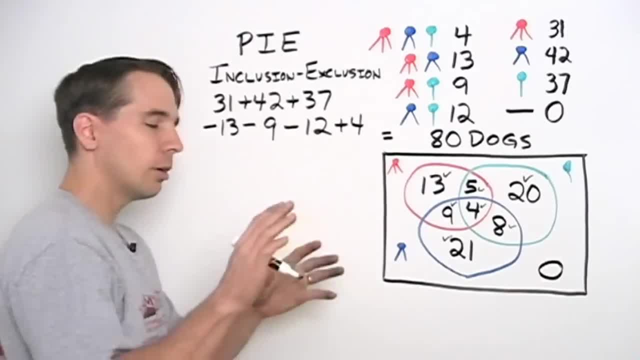 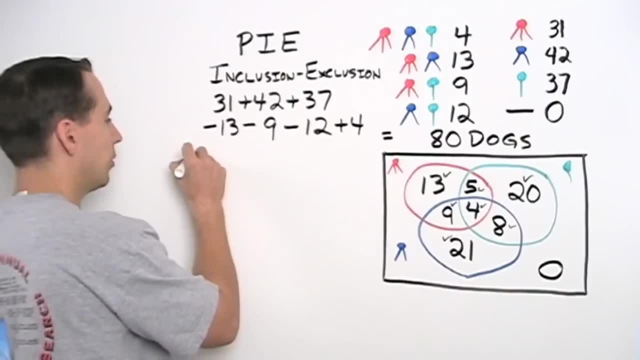 I'm like, oh, here we go with pi again. He said no, no, no watch. And he showed me. We start with the green dogs, dogs with the green ribbons. There are 37 of them, So we want the ones that have only the green ribbon. 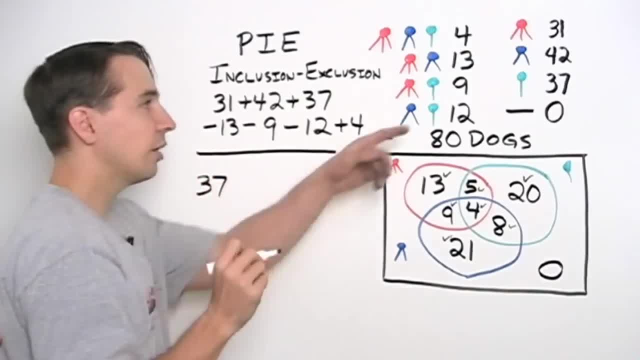 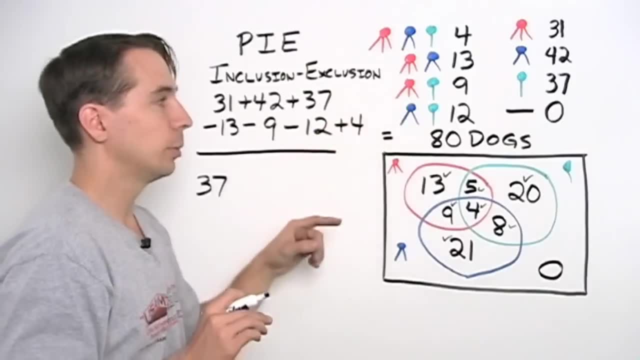 nothing else. So when we start with this 37, we're counting all the green ribbons, we're counting some of these other dogs And we don't want to include the dogs that got both a red and a green ribbon. We don't want to include the ones 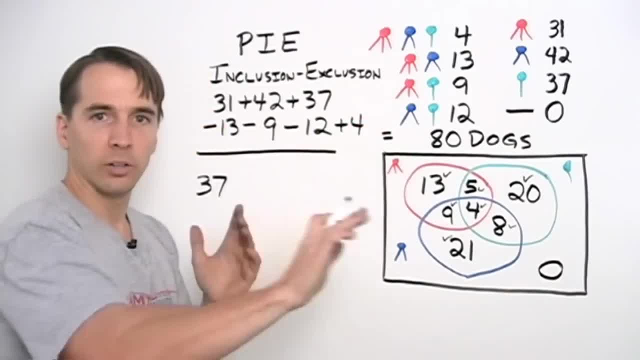 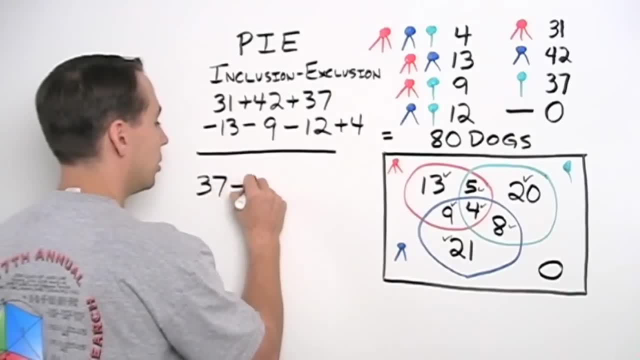 that got a blue and a green ribbon, So we got to subtract them. We're going to subtract them off because we don't want those dogs, We want only the ones that have only green ribbon. So we're going to subtract 9, subtract 12.. 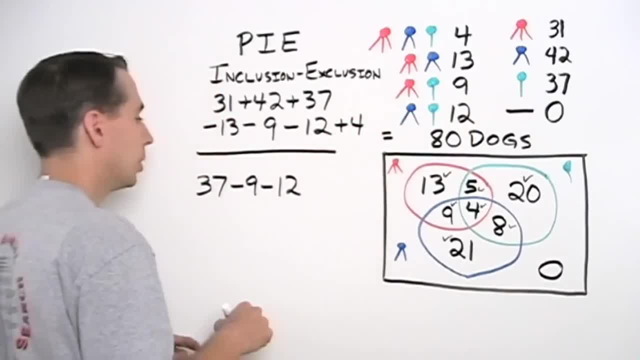 Because we want to subtract off these dogs from the ones who received a green ribbon. And I pointed out to John. but wait a second: 37 minus 9 minus 12, that's 16. That's not 20. You're wrong. 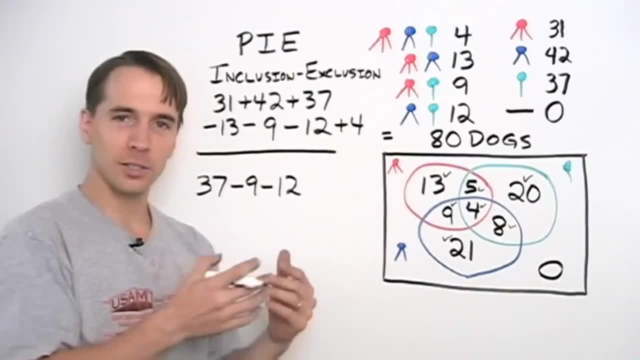 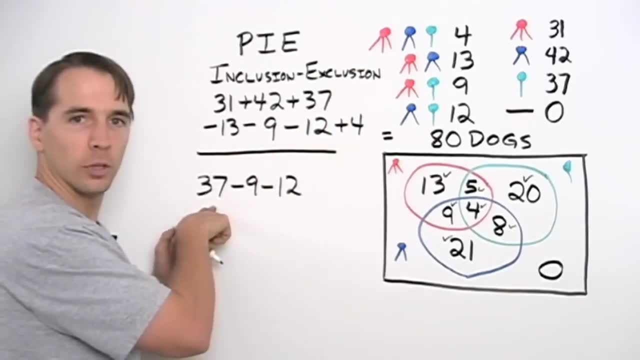 I said, hey, I forgot about the super dogs. The super dogs, I have to remember the super dogs. Let's look at what this count does with the super dogs. Well, I've added them once here because they received a green ribbon. 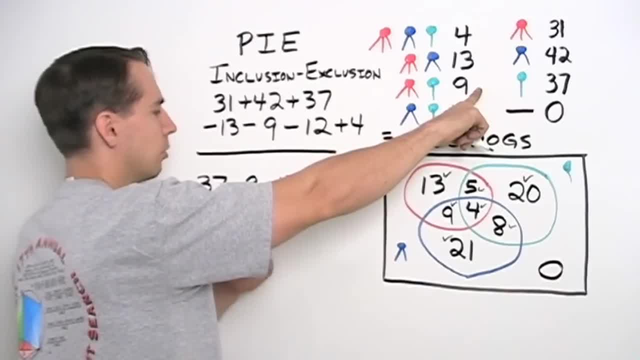 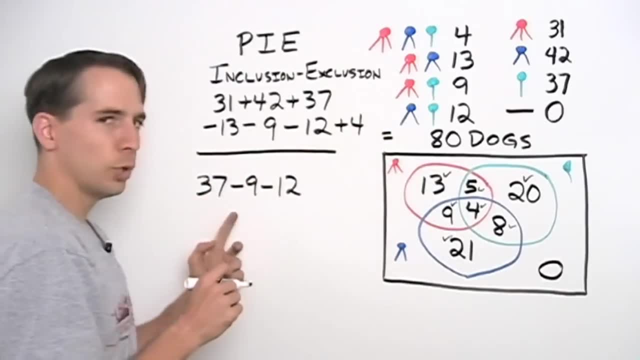 And I subtracted them once here because they received a red and a green. I subtracted them once here because they received a green and a blue. So I've added them once and subtracted them twice, But I don't want to count them at all. 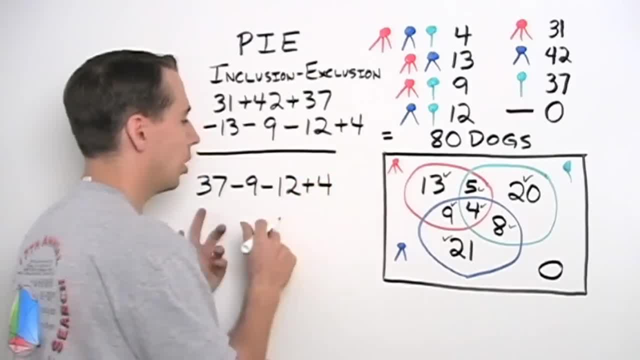 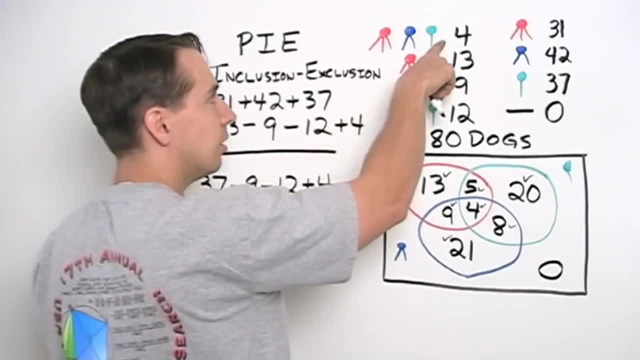 So I have to add them back in to make sure the super dogs are not counted and not subtracted once I've done all of these. So let's check this out again. the super dogs: I add them once. for the greens, I subtract them once. 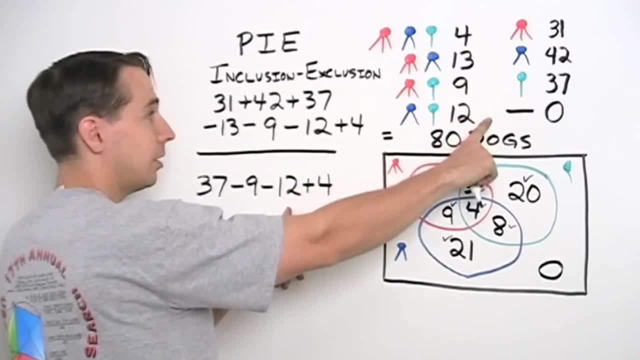 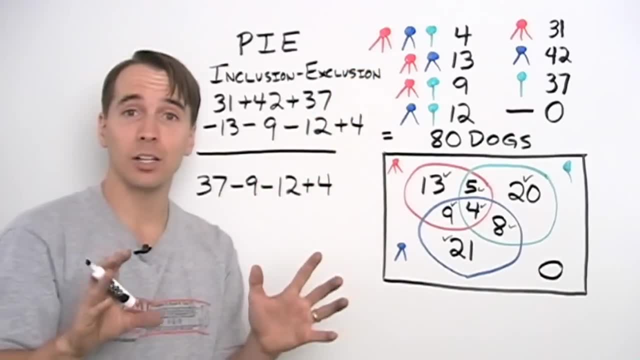 because they have a red and a green. I subtract them again because they have a blue and a green, And then I add them back in at the end. So now my super dogs are added twice, subtracted twice. they're not counted at all. 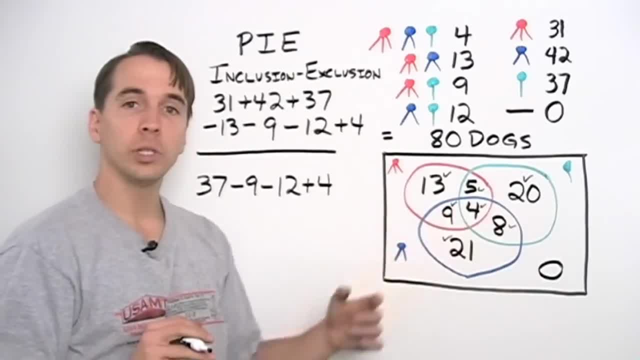 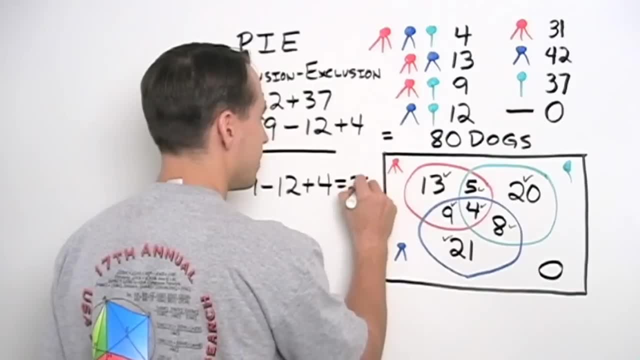 And that's exactly what I want, because I want the dogs that have only a green ribbon. And sure enough, 37 minus 9 minus 12, we saw that was 16, add back in that 4, 20.. And his subtraction method is pi.